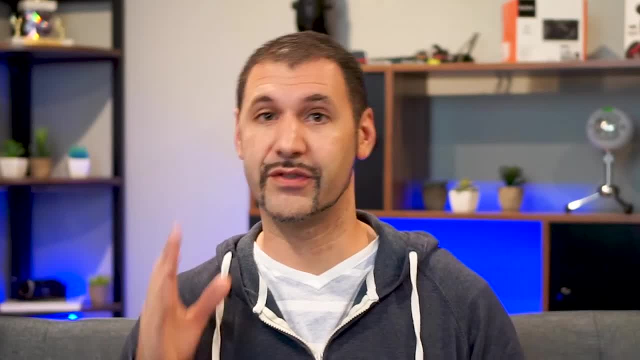 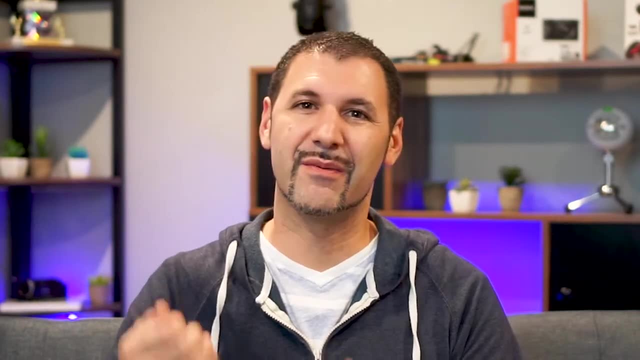 two states. So we're going to go over what different variables that you're going to want to learn and pick up to give you guys the tools to make the best choice. That way, ultimately, you can save the most money on your car insurance. Here's what I recommend you do: Grab pen and paper. 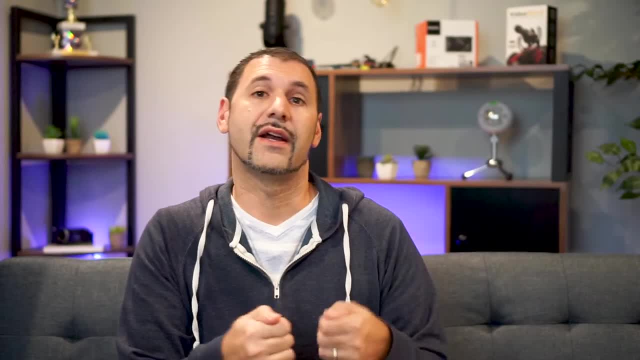 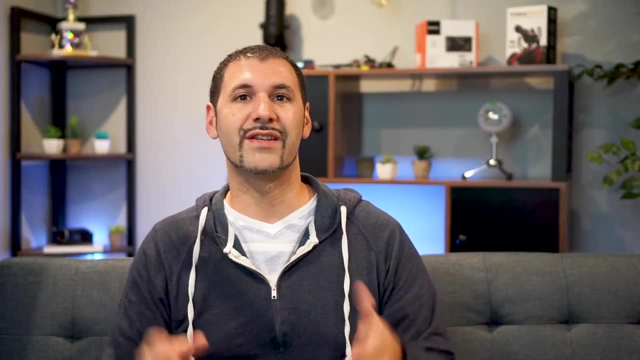 get out your notepad, tablet, iPhone, whatever you want. If you want to save this video, just click on the add to playlist and watch it later, if need be, But you want to make sure you write down at least these top seven things that we're going to go over. Do do me a favor, If you. 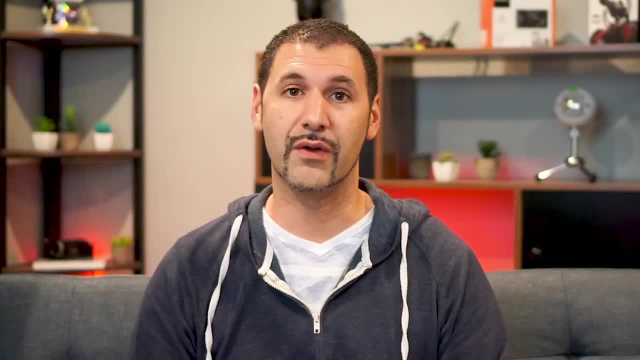 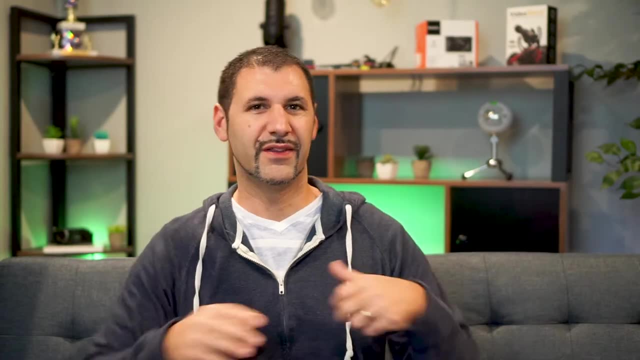 do get good value out of this. definitely share it with anyone that you think would also need this advice. But we're going to dive right into it. So the first part we got to describe is kind of what insurances are looking for. They're really just assessing risk- how much risk to how much. 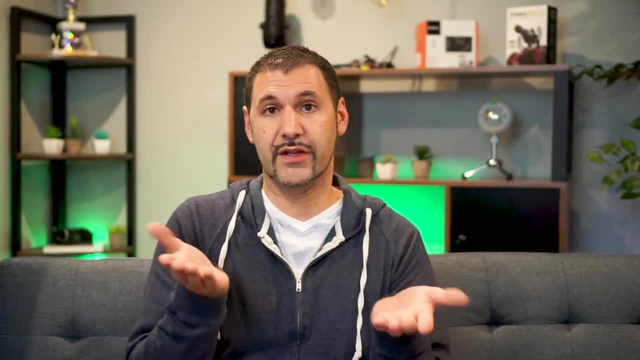 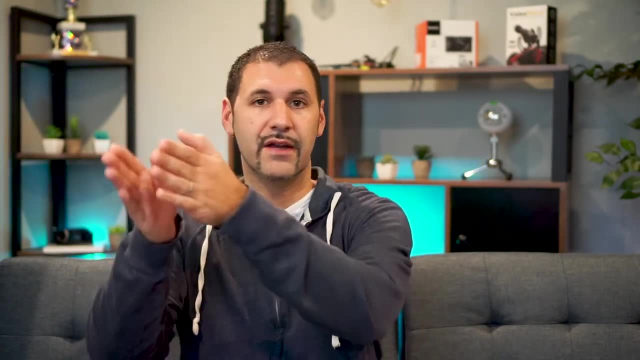 money we should charge And you may be a higher or lower risk. So you may have a ticket, you may have an accident, you may be perfectly clean, But there's different companies that are different fits for each of those avenues that you're at in life. So if you're the guy that has a ticket and an accident, 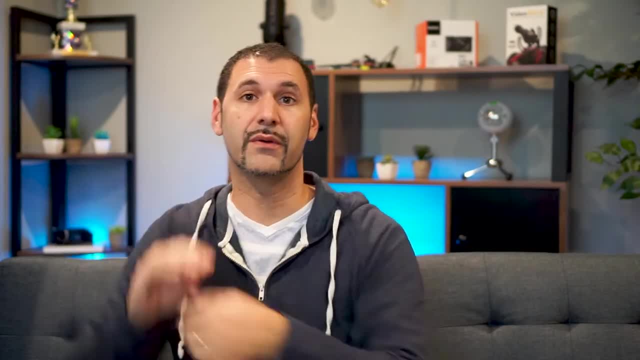 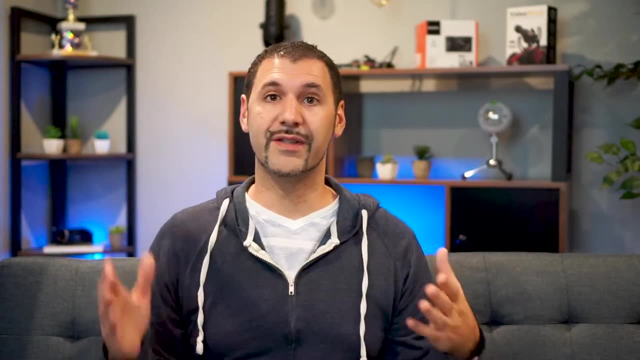 you need to go in this slot where these companies are going to be best priced for you Versus. if you're the guy that has a squeaky clean record, these other companies may be a better fit for you. Or you're the person that has a lot of money and you need to protect your assets, There are higher. level companies that are going to be better fit for you. So if you're the guy that has a lot of money, you need to go in this slot, where these companies are going to be best priced for you. Versus, if you're the guy that has a lot of money, you need to protect your assets. There are higher level. 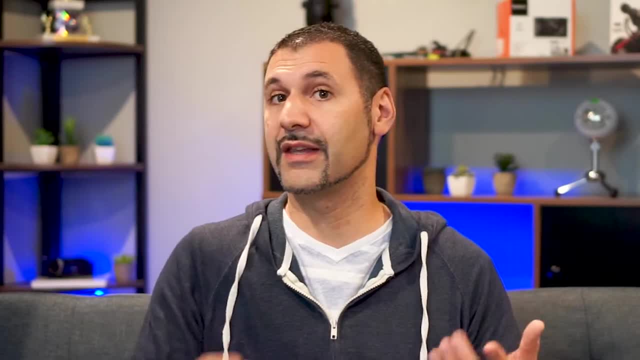 companies that are going to be better fit for you Versus if you're the guy that has a lot of money you need to protect your assets. There are higher level companies that insure those types of risks. You may want the person that wants better coverages. You may be the person that wants to have the best. 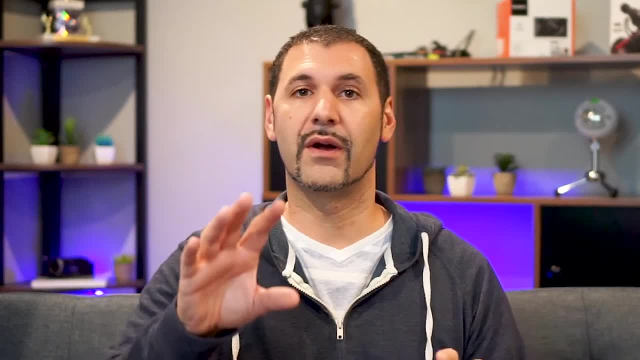 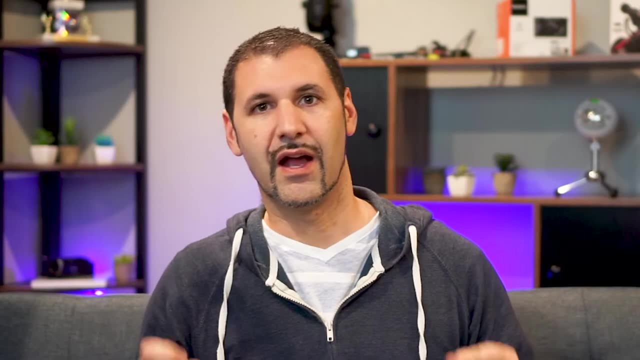 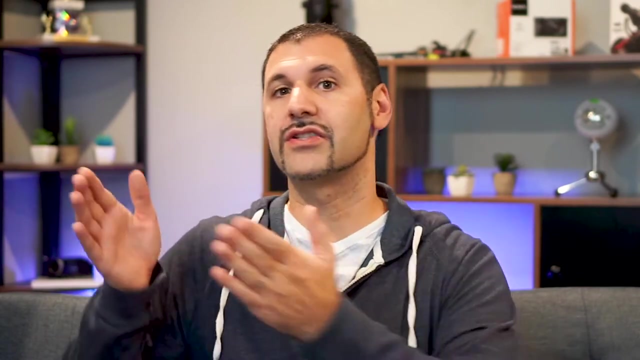 service That type of fit. there's different ones for you, And that's one of the reasons why these multi-agents, or they're called independent agents, are starting to spring up everywhere. It's one of the reasons they're more popular is because it's not just Geico, It's not just State Farm anymore. 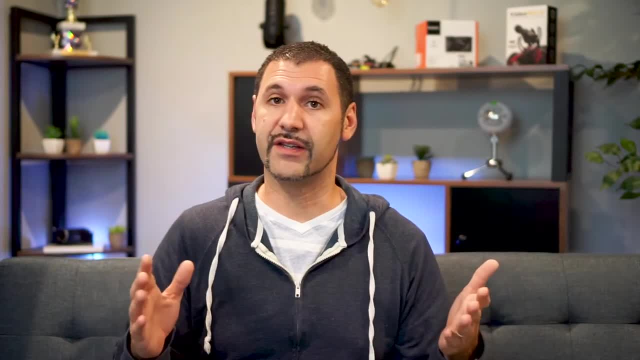 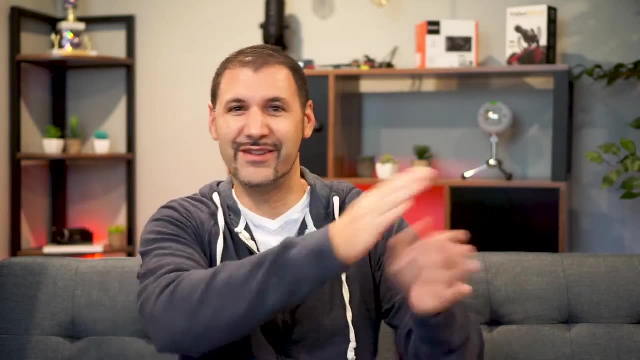 In today's age it's, one guy can quote 10,, 15, or, like the company I work for, 17 different companies at once. It's the kayak of insurance. You plug it in once they determine your risk and then up pops all these company options for you. 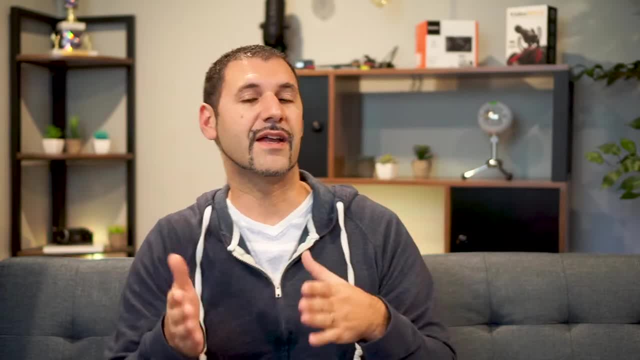 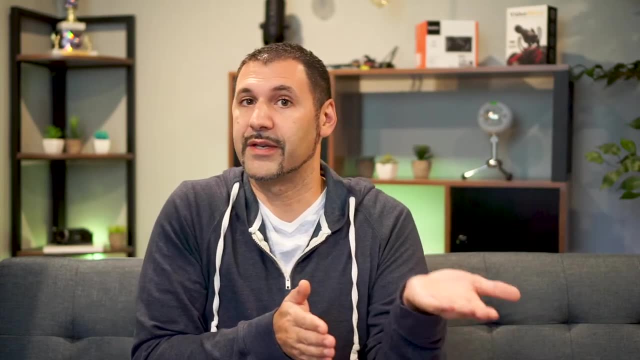 and they help you determine which one's going to give you the best deal. Now that agent's job is to kind of sift through that, because sure it may save you $10 more to go with this company A, but you're going to lose all these extra coverages that company B might offer. 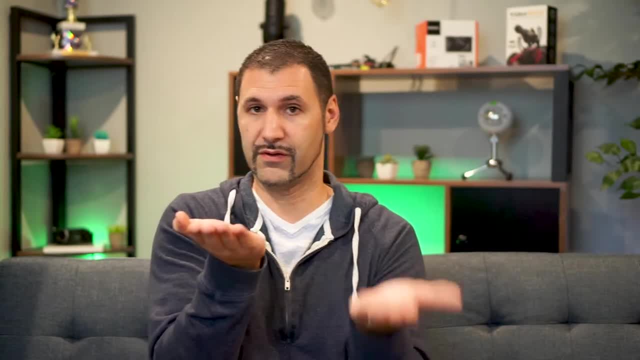 So it's their job to kind of say, hey, here's the best deal I can offer you, And then you're going to go with this company A, and here's your two options. If you're just looking for bottom dollar, company A is perfect. 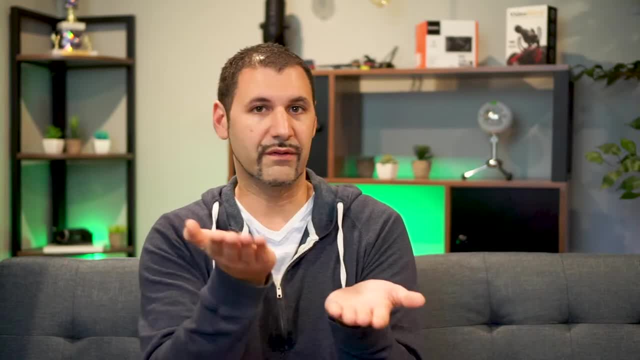 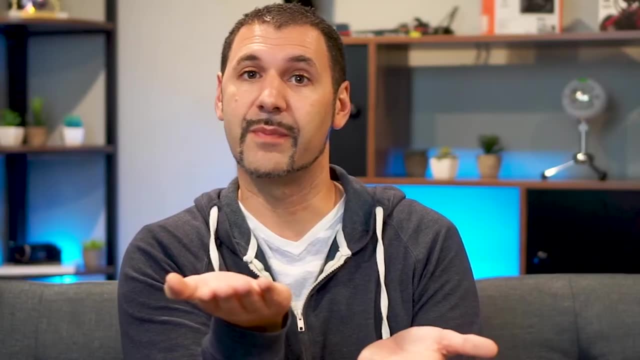 But if you don't mind spending an extra $10 a month more or whatever the cost is- might even be $2 a month more- then company B is going to give you a lot more benefits for the dollar that you're spending. That leads right into the very first point you should write down is what coverages 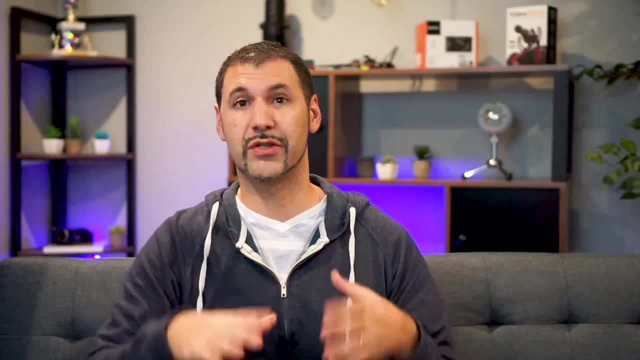 do I need? That's the first and foremost thing that you should determine right now. If you don't know, I'm going to link a video up to here. It's one of the first videos I ever made, Actually my most popular video. 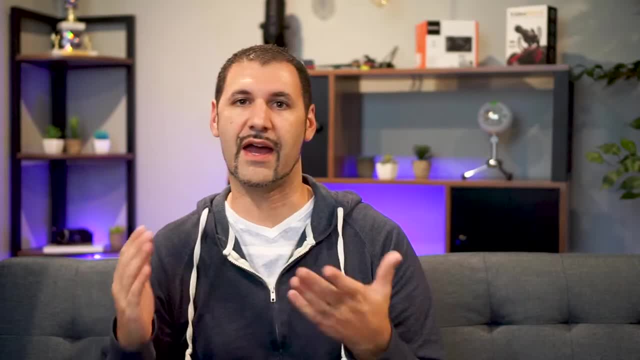 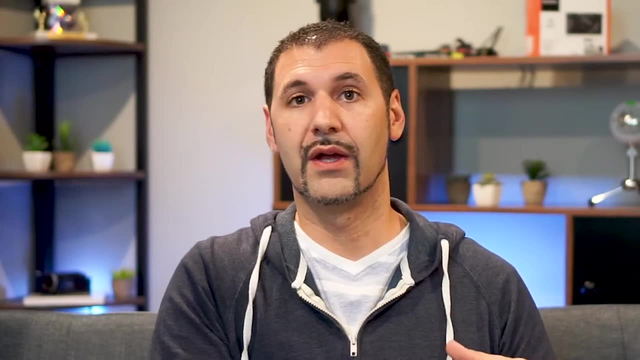 But it's very in depth on how to determine what coverages you need to have in car insurance. Determining the coverage you need should be the first thing you figure out, mainly because you want to know that these companies are competitive. If you're the type of person that likes to do the 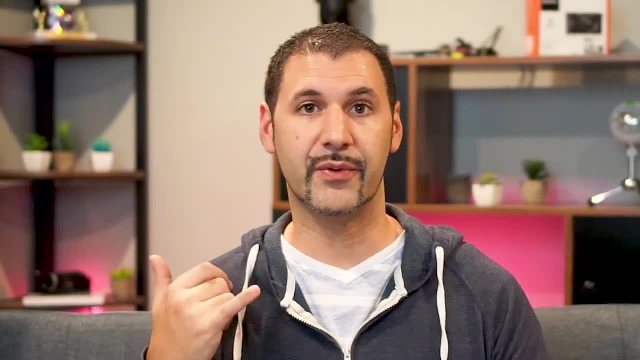 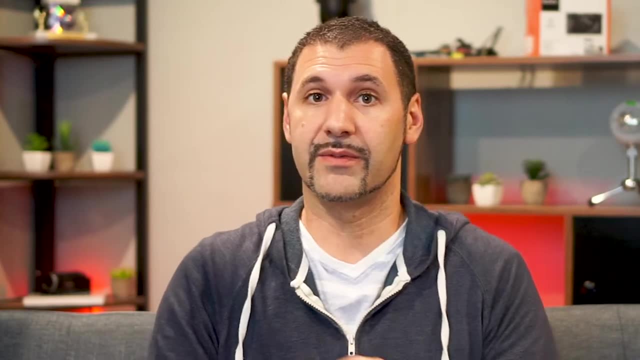 work and call yourself. make sure you're quoting apples to apples. You need to tell them: here's the coverages I want. Quote me based on those. Now, some people may only need the state minimums. Other people need to have those higher limits. Do you need an umbrella? What type of stuff do you? need to have. So determine that before you shop. Part of that coverage might be that you have a newer vehicle. If you have a loan on the vehicle, you're going to need to have full coverage. That adds comprehensive and collision. We're not talking about rental car road service. Those are additional. pieces, But when you have a loan they require that the vehicle itself is covered. That coverage can cost you twice as much. So you may have a $60 a month price, but because you have full coverage now, you're paying $120, $150.. It really just depends on that vehicle. And what type of coverage you need If you're new to insurance and you're just starting to drive. this is one of the reasons I say: buy a cheaper vehicle, get PLPD, personal liability and property damage and just get- just get a good coverage that'll cover the liability in case you hurt. 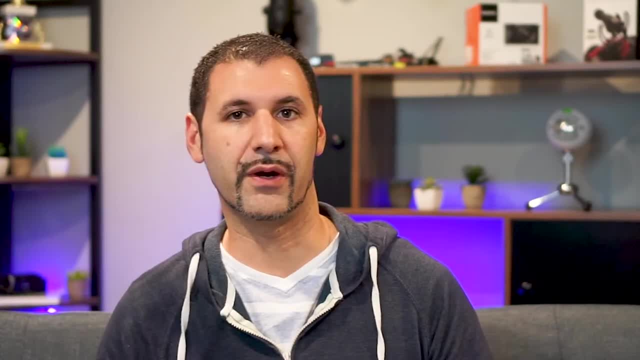 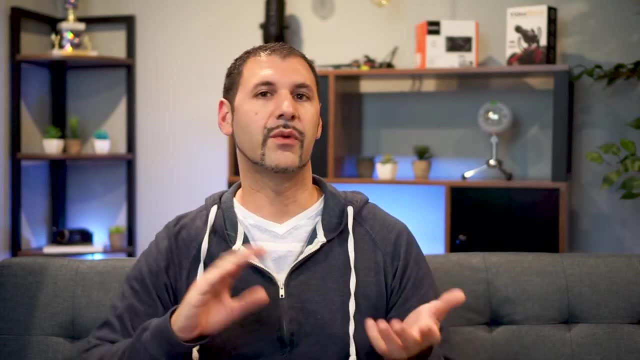 someone, But then you don't have to pay all that extra cost until you can afford it. The next part is where you live, the location. A lot of past insurances have done it based on zip code, And what's happening is a lot of these laws are starting to change where they're doing tariff. 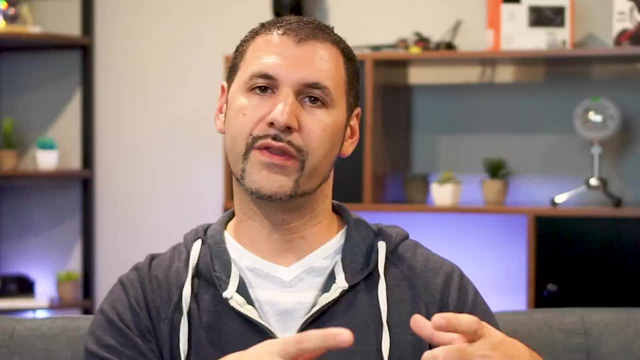 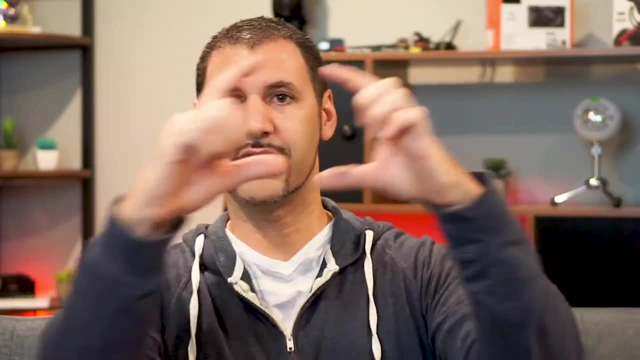 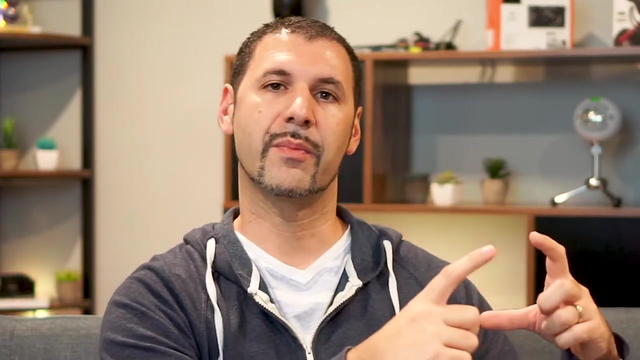 so it's like multiple zip codes in one territory. What this does is these companies take a look at it from a magnifying glass and they're saying, okay, out of all these areas in Michigan or Arizona or whatever state you're in, which ones are the riskiest? How many claims are we paying out? 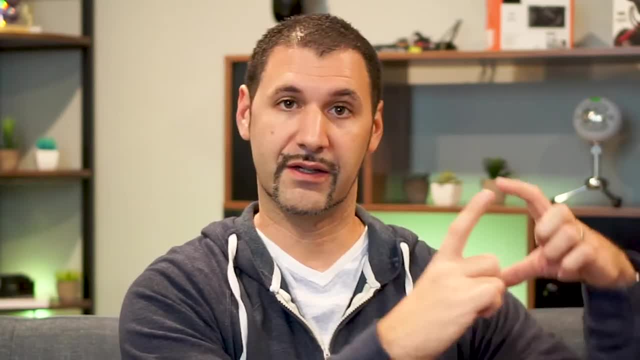 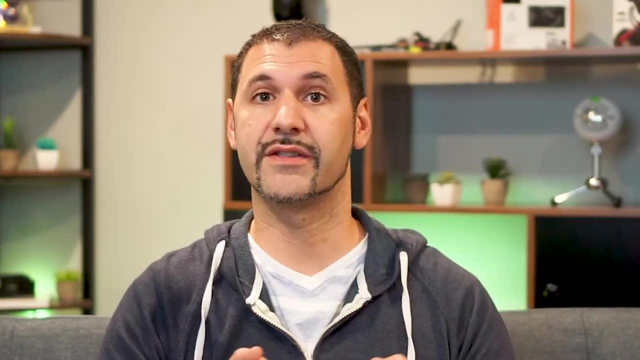 versus the premium that we're taking in. So if you're in this area and it's that red area where they're getting a lot of claims paid out and they're not taking enough premium, they might be profitable because all these other areas are taking in money. So if you're in this area and it's 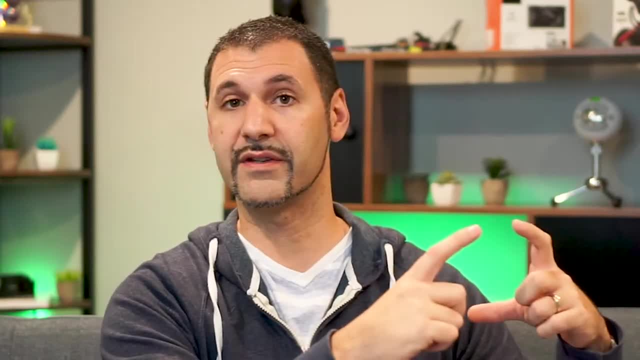 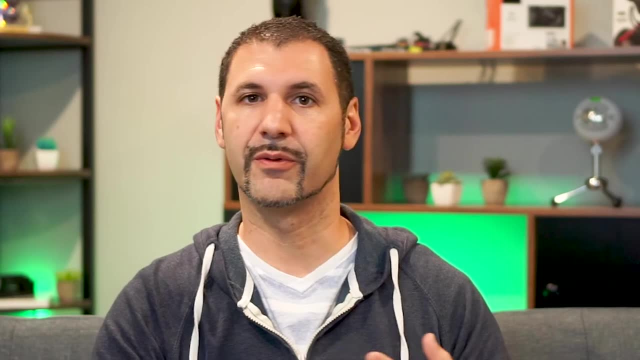 not having claims. but that area that you're in, or whoever's in, is going to pay a higher price because there's more uninsured motorists, There's more claims, It's maybe more congested and a lot of people are filing insurance claims. There's more theft and vandalism. That makes a big 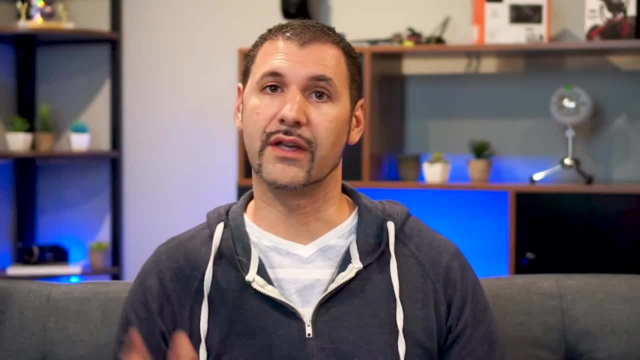 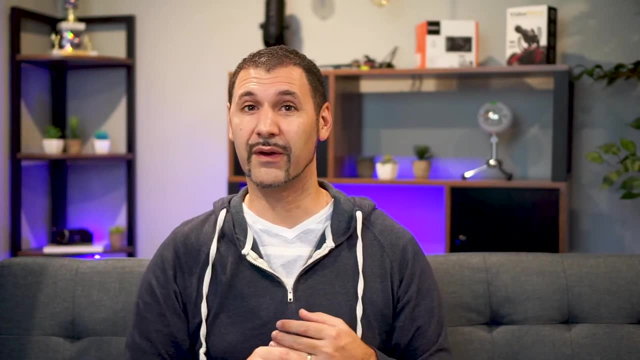 difference on the premium That would be. the second piece is just knowing the location that you're in. Number three, your driving history. Even if you haven't had any tickets or accidents, you actually might be in this category. Let's start from the beginning If you do have accidents. 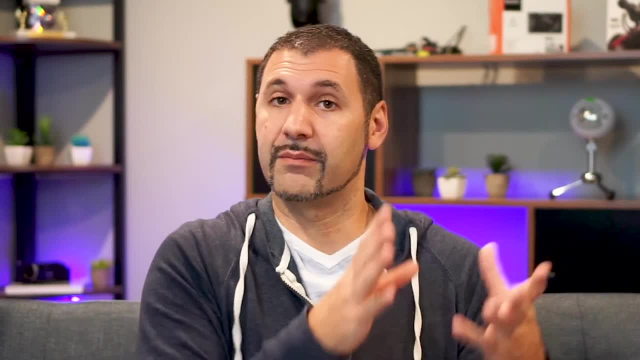 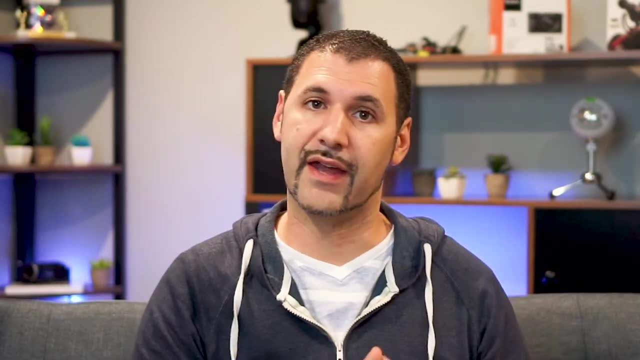 and tickets, then yes, that makes a difference. But, like I said before, there are companies that are perfectly okay with one or two tickets. There are companies that don't mind having an accident. There's companies that freak the crap out if they see you have an accident. For those of you that, 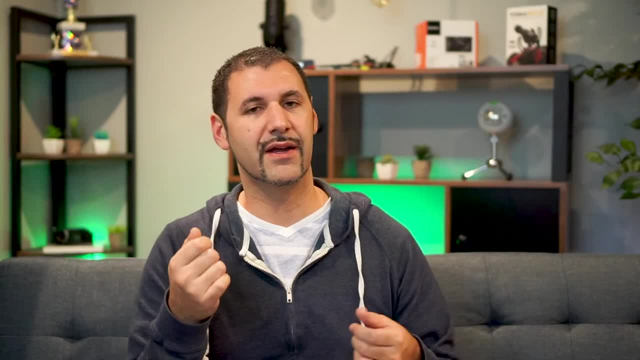 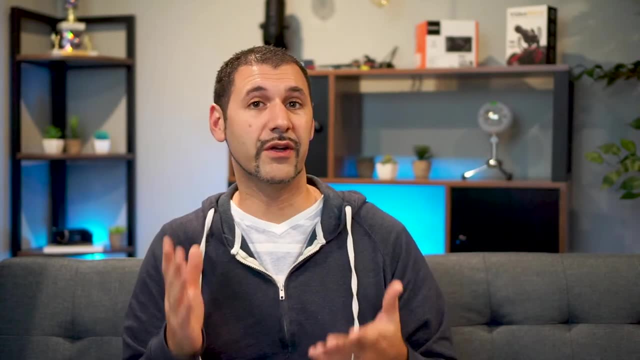 have a perfect driving record. if you're noticing that the rate seems high, ask the person that's quoting you or your agent if they have anything on your driving history. I've actually had quite a few times where I go to tell somebody the rate and they're like: oh, I don't know, I don't know. 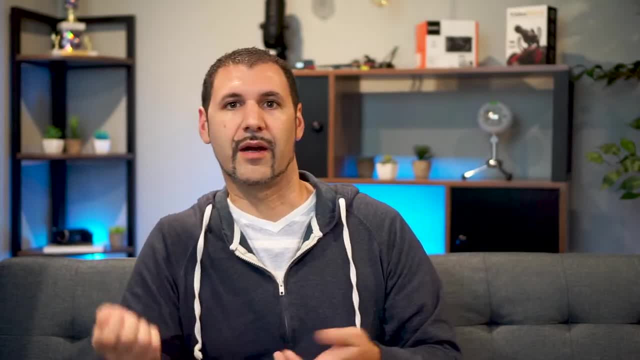 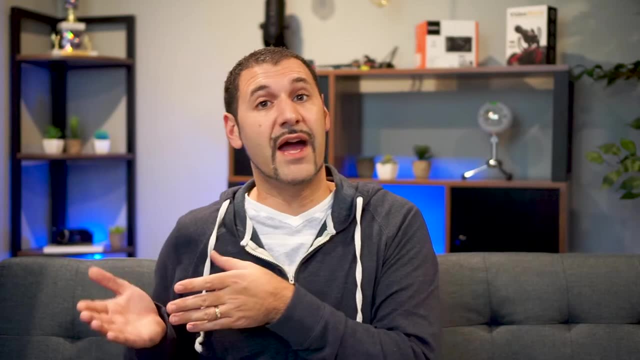 They're asking me why it's so high. I explain to them. well, you have a comprehensive claim on your driving record or you have an accident on your driving record. You may have been involved in an accident as a passenger, You may have been in no accidents and somehow something's showing. 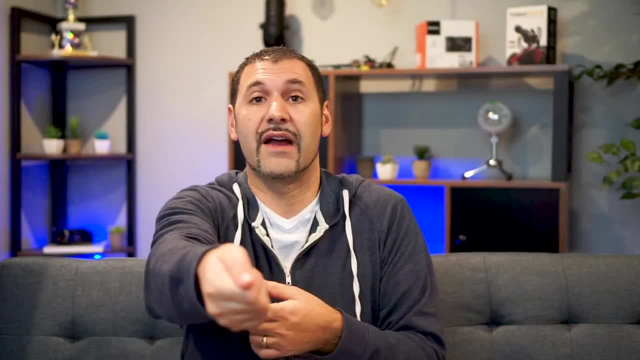 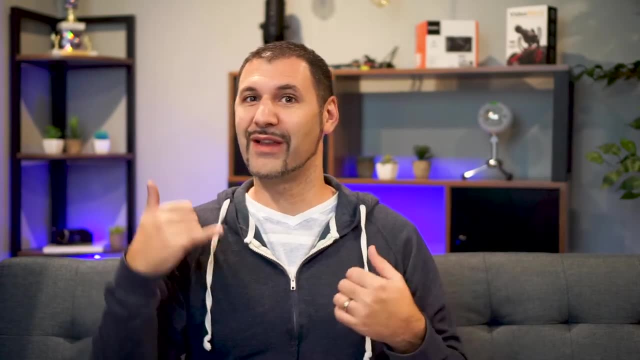 up on your record. You may have even been in a fender bender and gave the guy $500. He went his way, You went your way. He called his insurance and actually told them that you hit him. There's a lot of different ways that this can happen. Just be mindful of that stuff. Anywhere from three to five years they will track back to. If it's not yours or it wasn't your fault or you're not the driver, it's very easy to get those removed. The agent just has to talk to the underwriter and just explain the situation. Those of you that have had tickets and accidents, if you've taken a defensive, 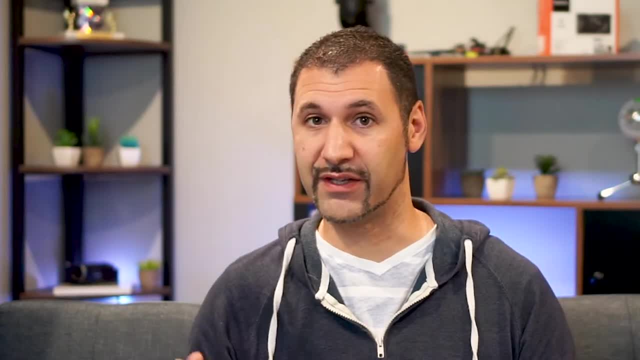 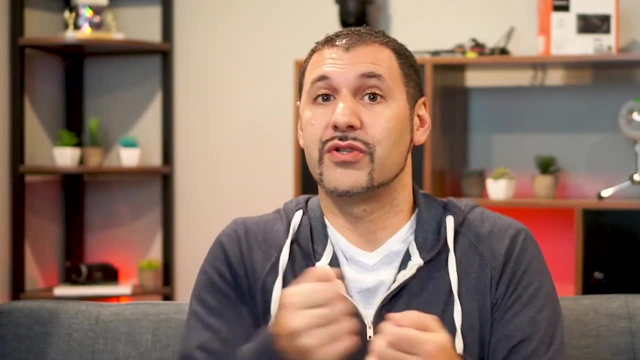 driving course. keep in mind that doesn't remove it from your driving history, It only takes the points away. So when the state looks at your points and says how many do they have, You may have zero. but you might get a higher price when you go to insurance because it doesn't come off. 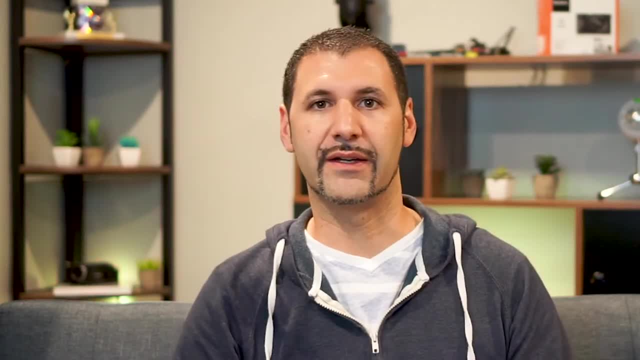 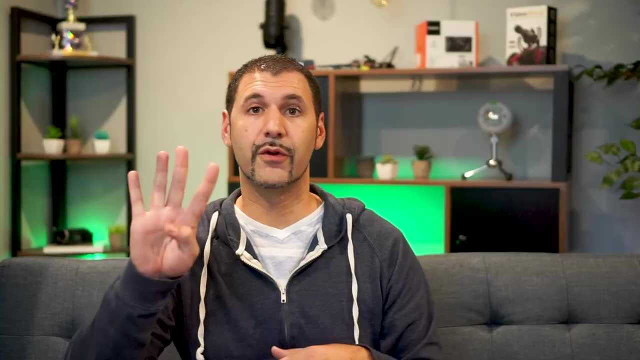 your record. There are a couple states, such as North Carolina, that does offer what's called a prayer for judgment, where it does completely remove it from your record, like it never happened. The fourth piece is the number of drivers. This is in your household, So when insurance is rated. 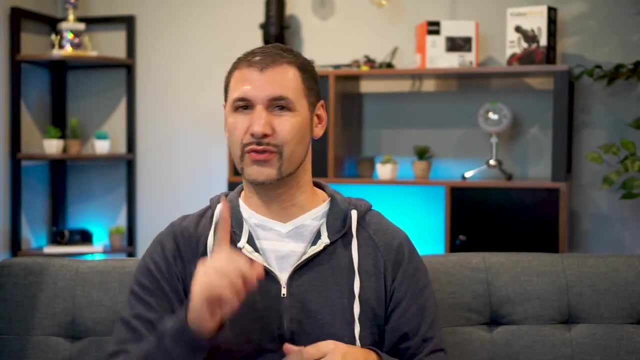 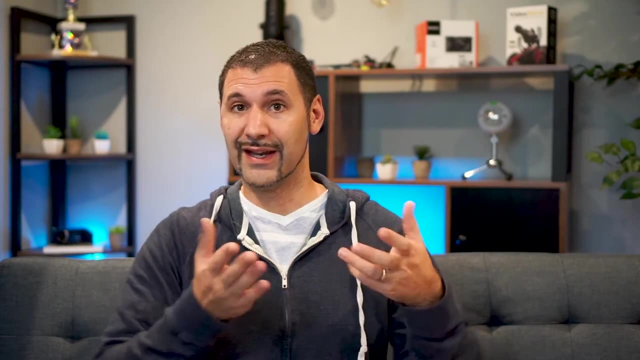 it's usually rated in a household, not just one individual. You may be the only person that's going to be on the policy, but if you live with four other people and two of those people don't have insurance, that's a risk that they have to take on. Is Jimmy going to drive your car, Is he? 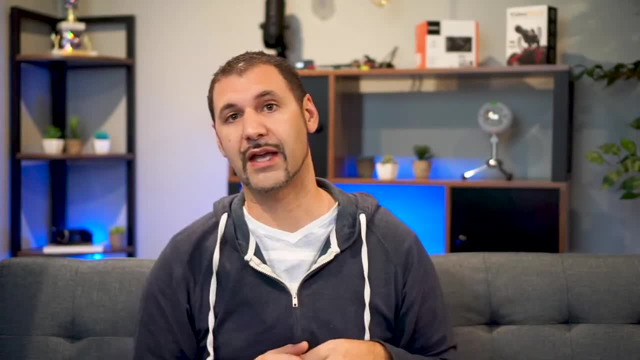 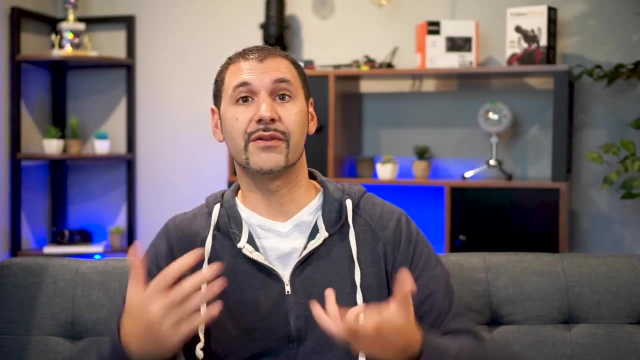 going to give the keys to Susan to go to the gas station? What if Bill needs to leave for work and you've blocked him? What if he backs it out and hits something? They have to pay those claims because they're insuring the car if you're doing full coverage. but that's a risk that they have. 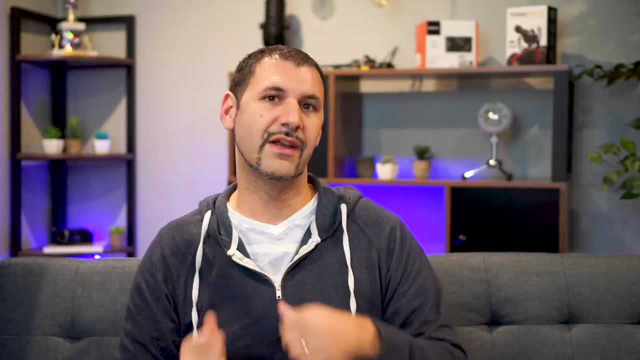 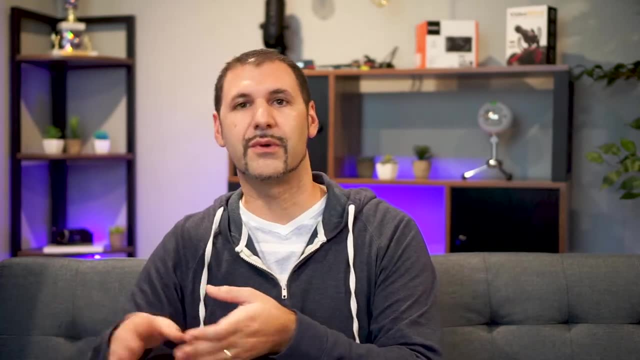 to determine. In most cases it doesn't make a big difference because usually they have their own insurance. You just tell the agent and the agent usually just puts down two other drivers in household has their own insurance. There are some companies that rate for that. So if 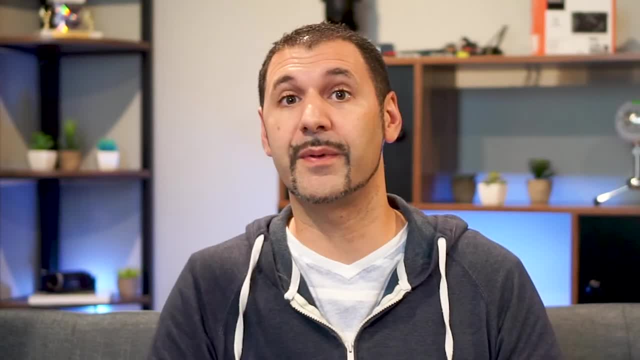 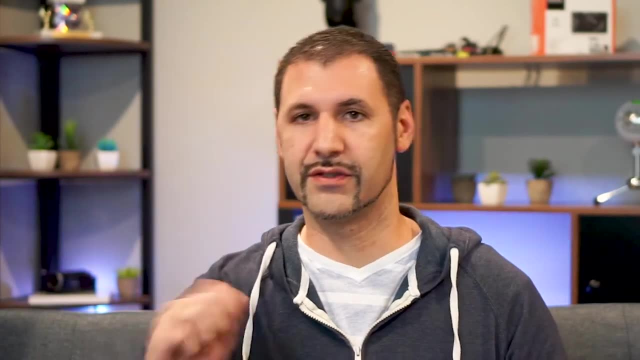 they're best friends in the house, even though they have insurance. some companies actually charge for that. You can't exclude them. So that's an option. You're going to say they'll never drive my car and they'll just sign a piece of paper saying Jimmy's never going to drive my 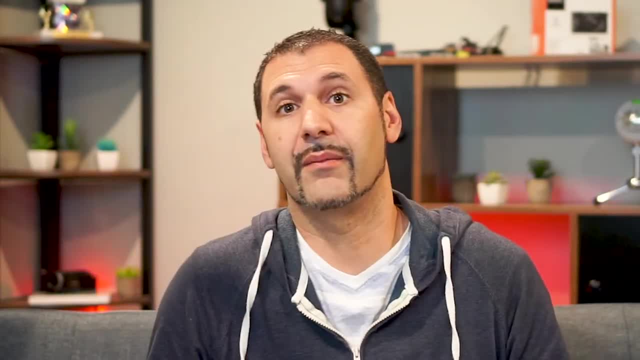 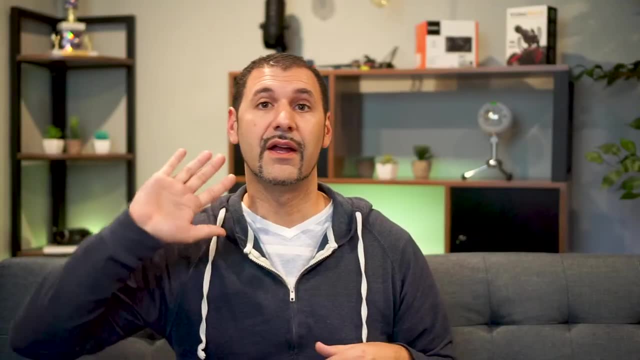 car. If he does and he gets in an accident, they're just not going to cover it. That's the fourth piece of: just be mindful of how many people are in the house and whether the insurance company even cares. Piece number five: your age. It plays a big factor. We're not going to go too in depth. 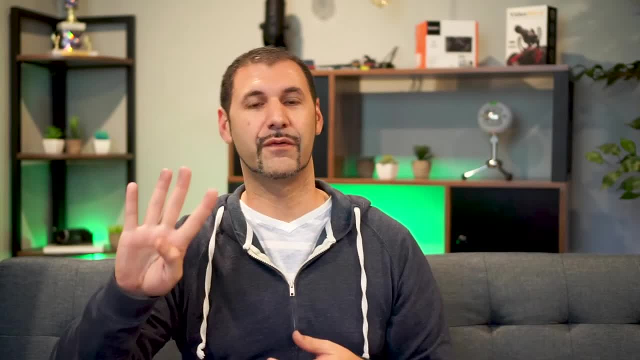 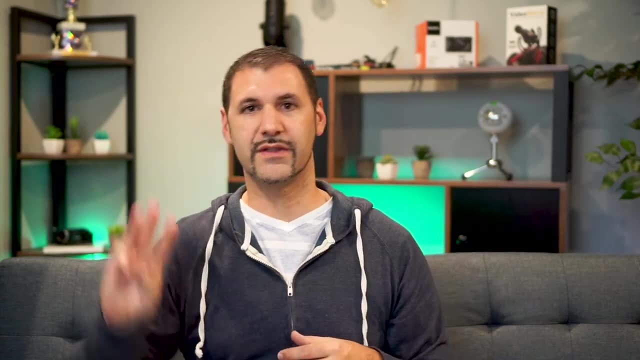 with it because you can't control it, You're, however old you are. today There's four age groups to know, So it's 15 to 25.. If you're in that age group, that's the highest risk. There's 25 to 50,, which is the second best risk. There's 50 to 75. And that's 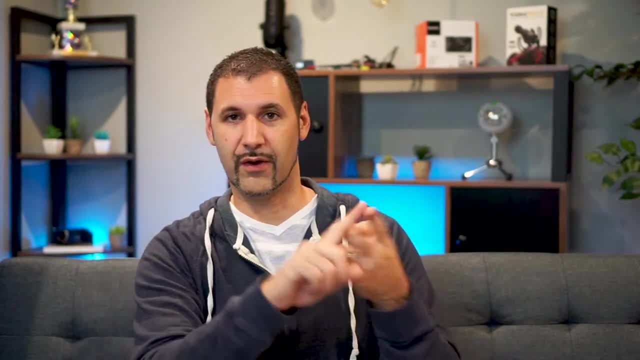 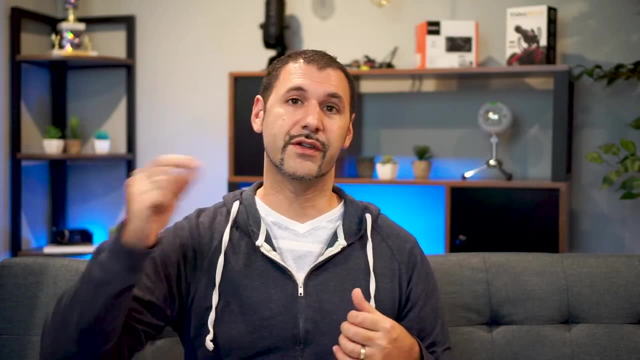 the best, the sweet spot. They call them confident planers. If you have a home auto, want full coverage and you're 50 to 65,, 75, and then there's 75 and above, where it starts to go back to a. 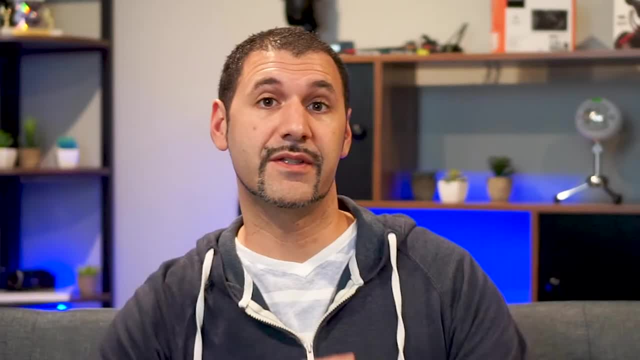 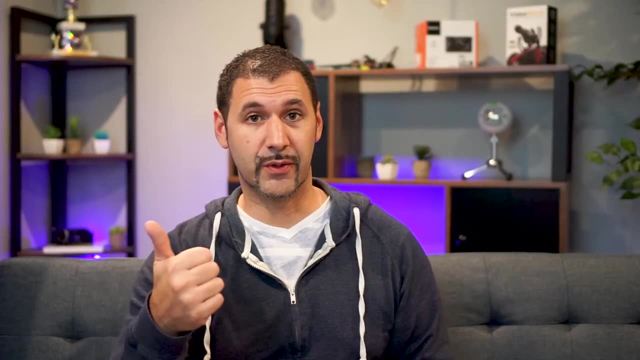 higher risk. The most important piece of this whole thing is tip number six, and that's the agent that you work with. There's a few things you have to know about your agent. Are they knowledgeable? Do they know what they're talking about? We work with 17 companies- Not everybody. 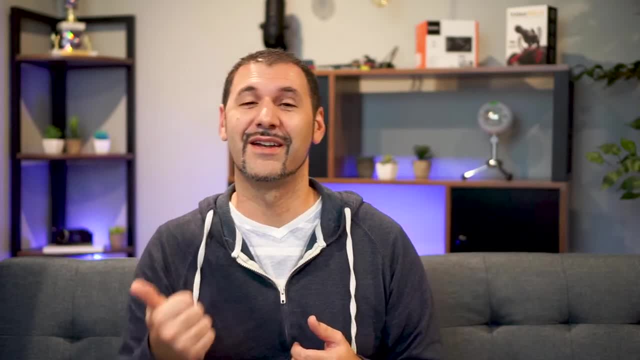 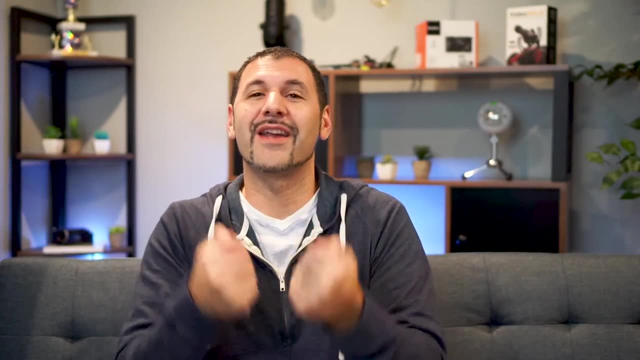 knows all 17 rules. of every company there is, There's 10 companies. they might work. They might even only work with two companies, but you would be surprised how stupid some agents are. They just want to sell you the bottom dollar. They don't ask you questions about your coverages. That's a. 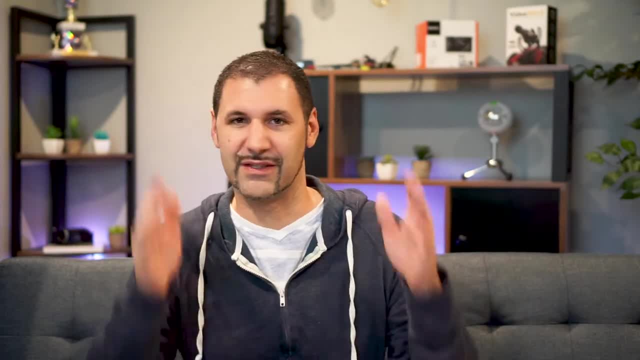 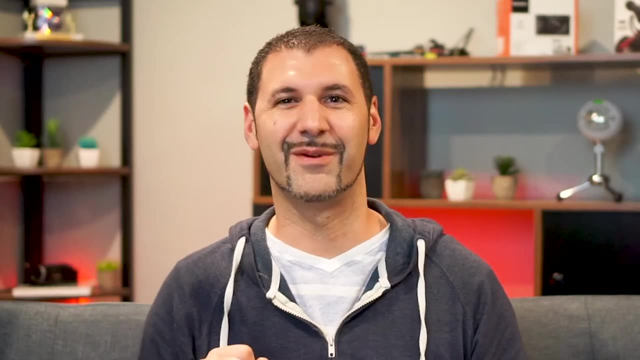 quick way to find out if they don't care is: they don't ask you anything. They don't ask you any thing, They just quote you a price. Do they know all the discounts? That's one of the things I prided myself on being. I was called the discount guy at my job because I knew every discount there. 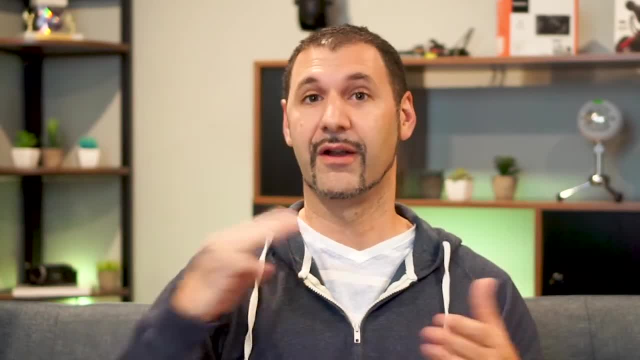 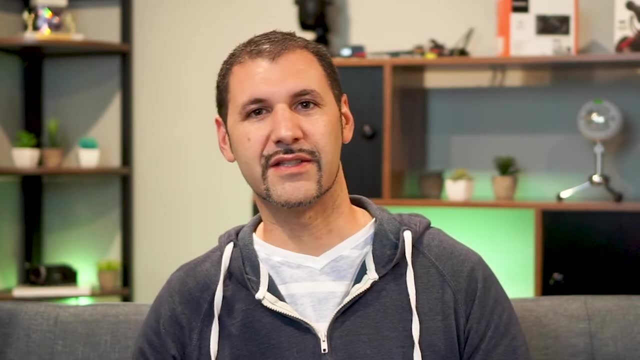 was Do. they know what benefits and coverages are better for each company? They're going to give you the best deal but also give you the most coverage for that deal. The easiest way to determine if your agent is knowledgeable: usually if they've been established for a year or longer in their 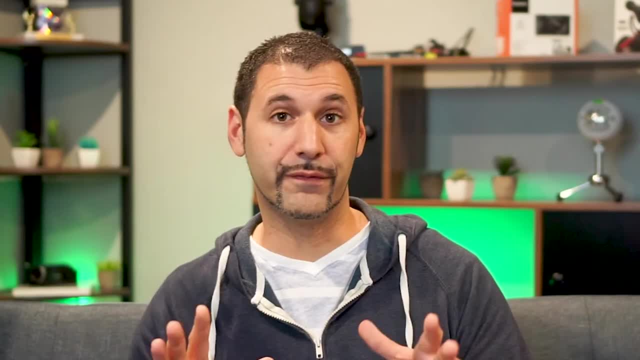 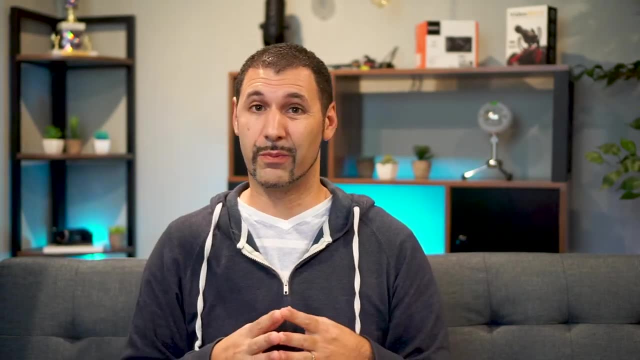 current position, then they usually know what they're talking about. Hopefully you can look them up online. Just Google the company. Look at the reviews. If they have lower than four stars, they're not the company that you probably want to work with. If you're just looking for the bottom dollar, sure they might be the fit for you. 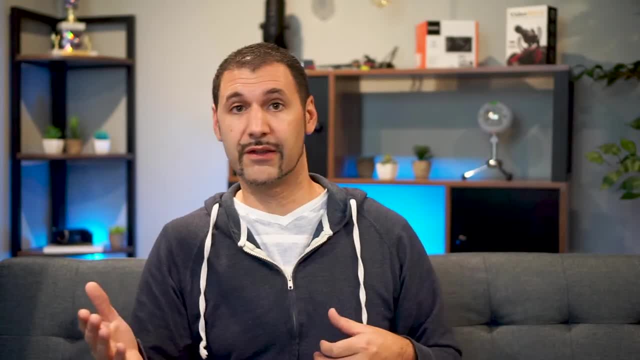 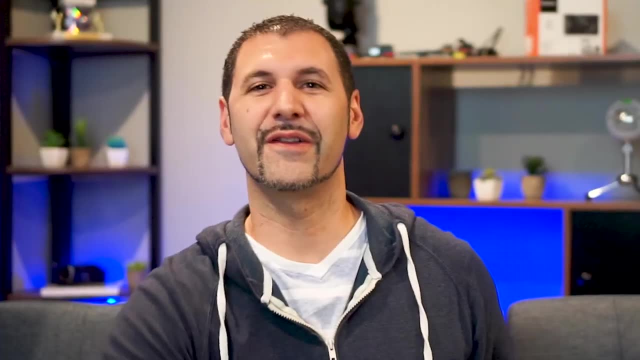 If you're looking for that guy that's going to fight those claims with you and help you get through a lawsuit and help you get through anything that you're going to have come up, you may want to tweak it to the four stars and above. I know what you're all thinking: How many. 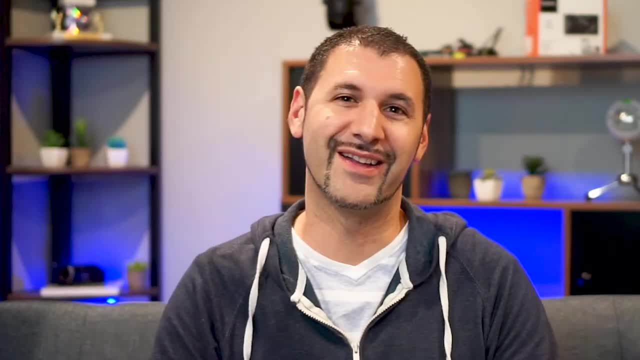 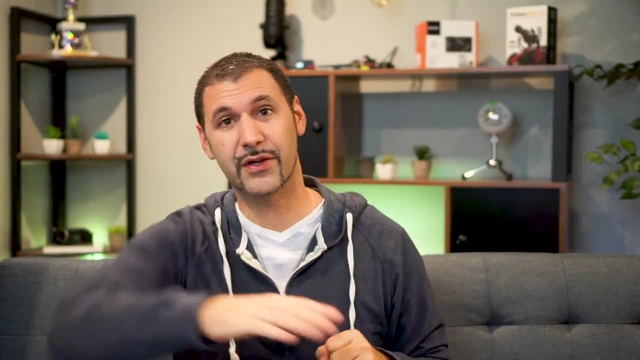 stars does the company he works with have? We're at like 4.9, so yay for us. The final piece is number seven. combining your insurance- And I'm not just talking about home insurance- Sure does that give you the biggest discount.